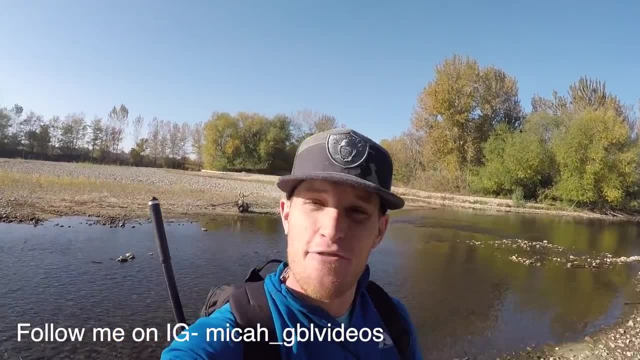 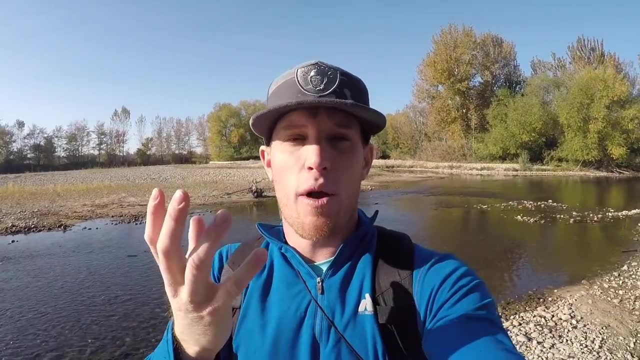 What's going on YouTube? fam Mikey here shooting another high adventure video. Guys, beautiful fall day. We are out here on the river again chasing big old brownies. I am in a little warm weather pocket right now, before it's supposed to get really rainy and cold. 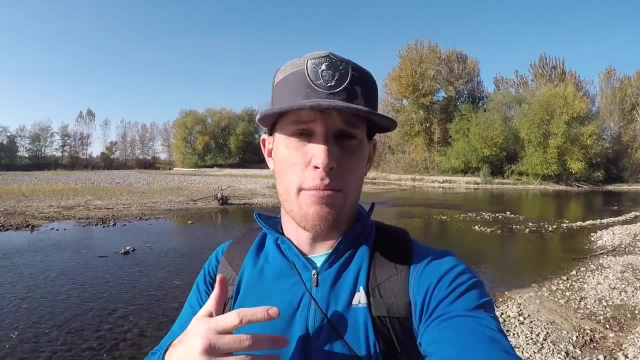 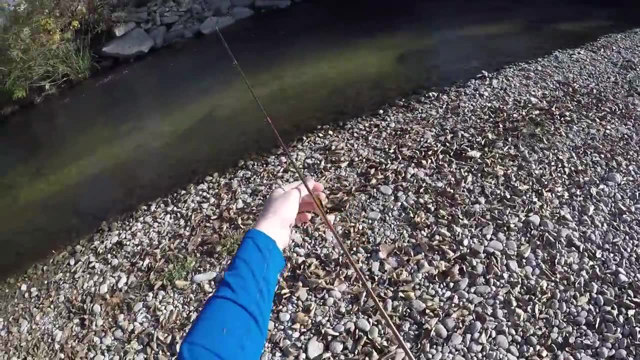 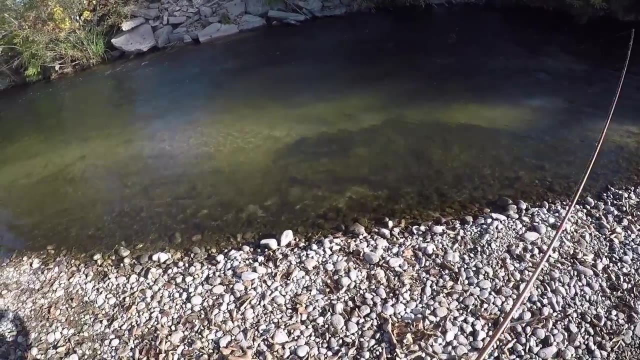 so we're at the river. We're gonna see if these brown trout are still in spawning mode, still super aggressive, Let's just get fishing. Oh there's one. Oh, it just came right up. Oh, there's a little. I don't know what that was. 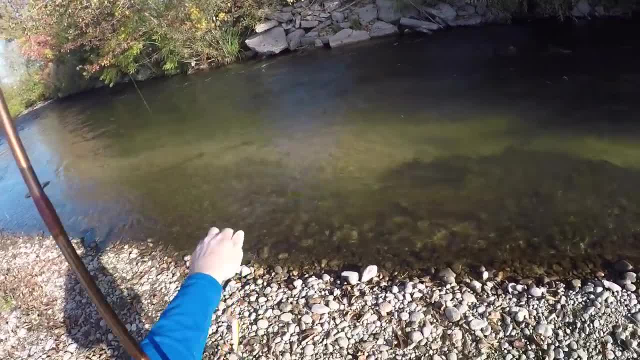 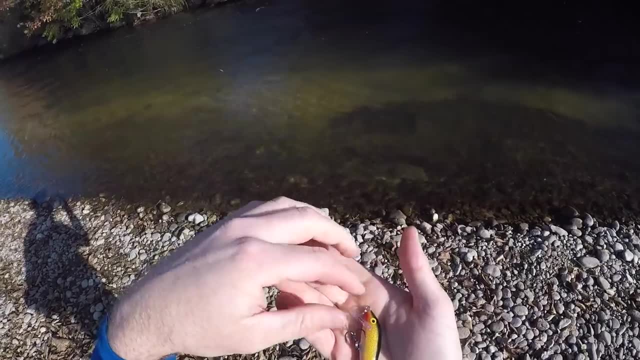 but it came right up and nailed it. Second cast of the day. Guys, this is what I am using as bait to start the day off with. Check it out. Nice little jerkbait golden color. I like those colors that mimic what a brown trout looks like. For whatever reason, it seems like they really. 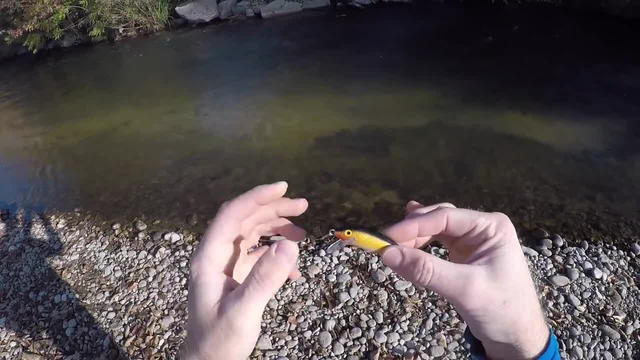 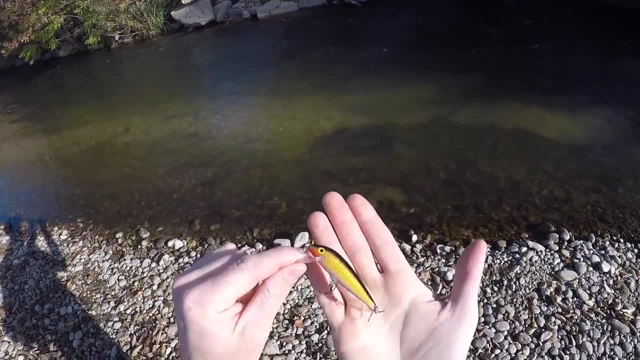 Cabela's or Sportsman's. I'm sorry, Cabela's or Sportsman's, I'm sorry, Cabela's or Sportsman's, But they're just too expensive. You can get the same exact thing, this bad boy, right here, for literally $1.50 to do $2 cheaper at Walmart. So there's your. 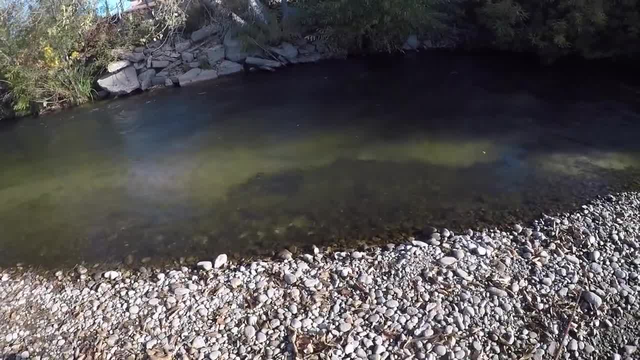 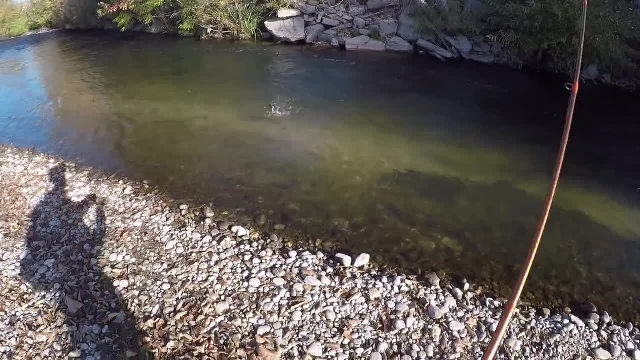 little helpful tip of the day. This is such a tiny area, but what this jerkbait's able to do, unlike the flies- is it actually gets down in that water like that, And I think it's able to get down close to those fish. This is a brownie to start the day, Guys. 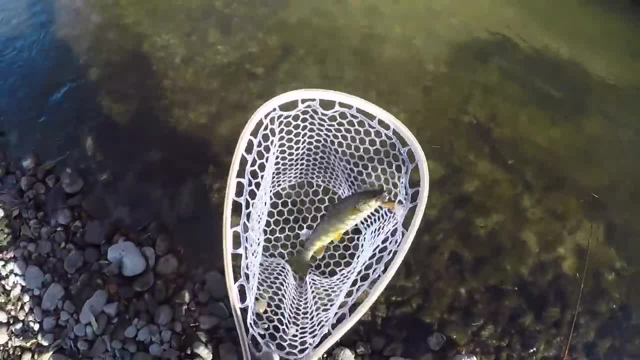 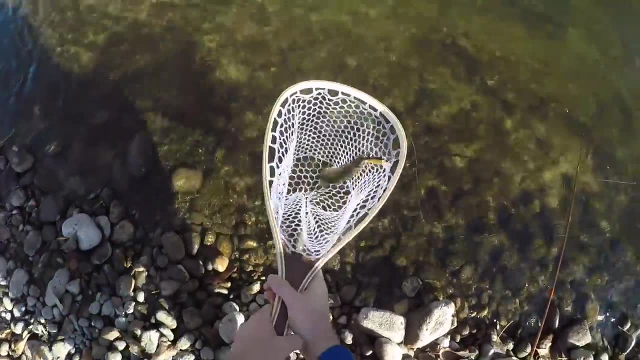 literally third cast of the day, And it gets down close to those fish and I think it just, it just is able to go right by them. Look at that. Look at that, It just swims right by them and you're able to nail them. Look at that, guys. Still plenty aggressive, it looks like. 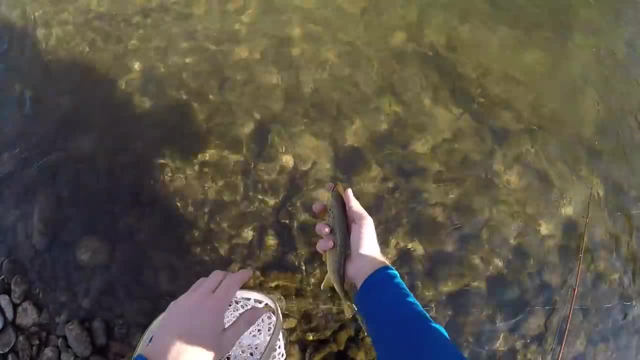 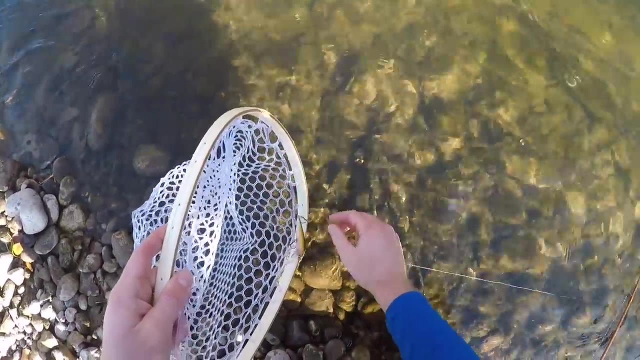 That's probably about 10 to 11 inches. Pretty fish. We'll get her back in the water. Literally, guys like my third cast of the day, Woo Perfect, This is looking like it might be a really good day. 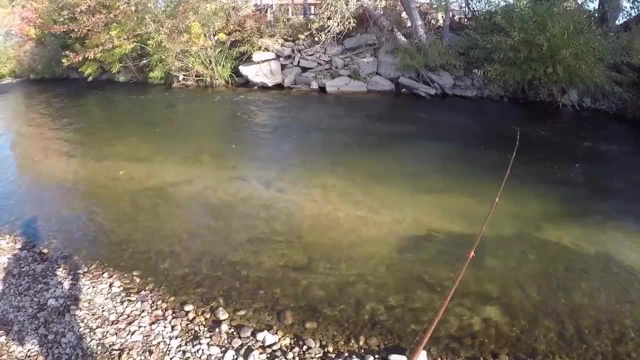 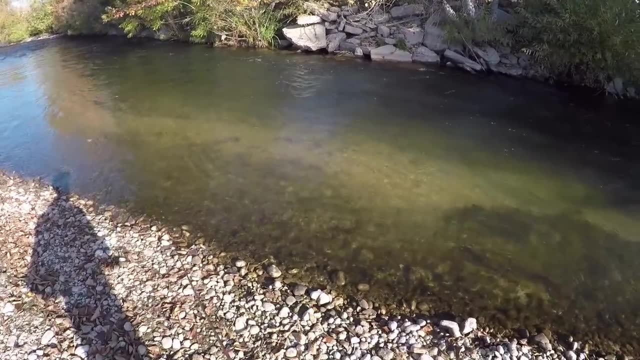 Literally just the first spot I pulled up on. It's nice and deep on the other side That jerkbait gets right down to their level. I just I love it. I think I just saw another one. No kidding, I think I just saw one following it up. Jeez, Louise. 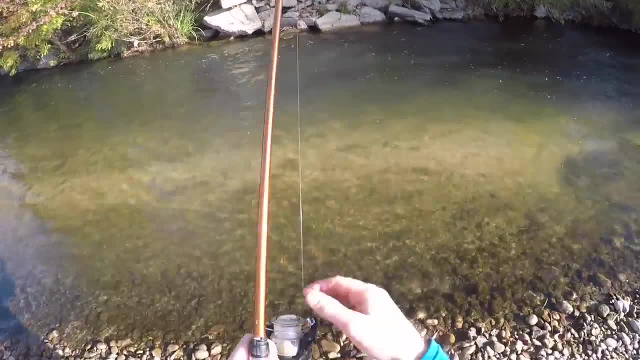 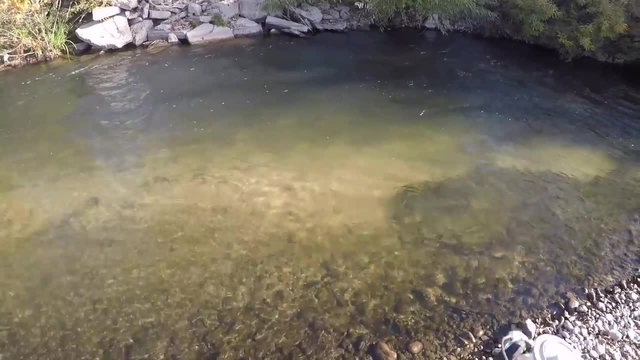 Oh, there's one. Oh, this is a nice one, This is a good brownie, guys. Oh, just came up and nailed it. Just came up and nailed it. I saw it. Oh, she's running all over the place. Look at this. Oh, this is exactly what we're after, guys. 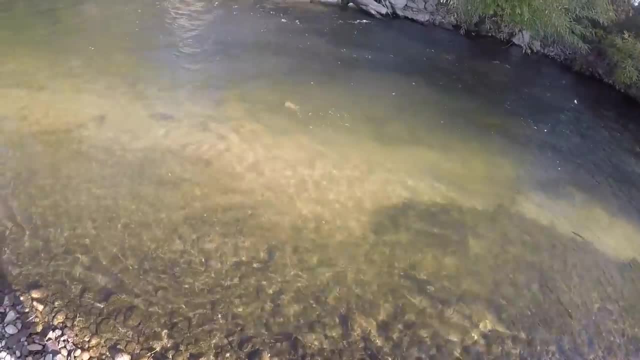 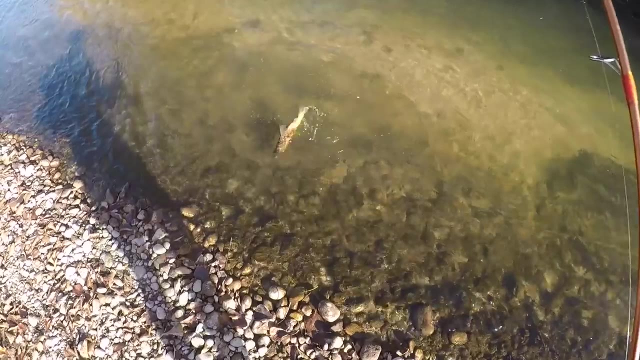 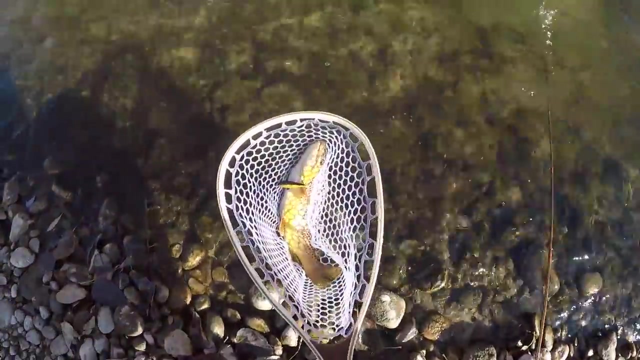 Look at this fish. You guys are going to love this. You're going to love this. Look at this beautiful trout right here. Looks like someone is still fairly aggressive. Oh look it foul hooked it. Look at that. Oh look at that, Guys, she swung at it and it hooked her. 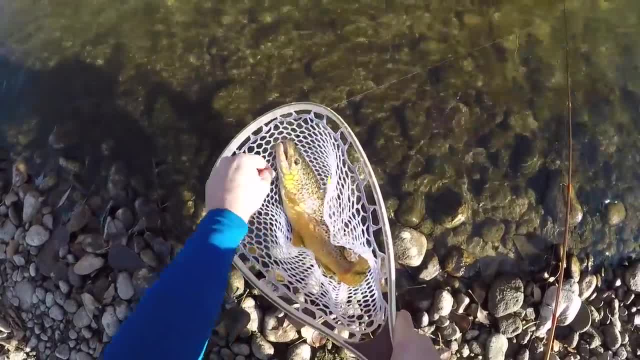 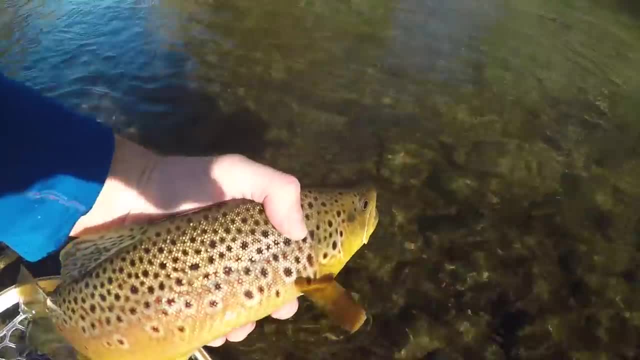 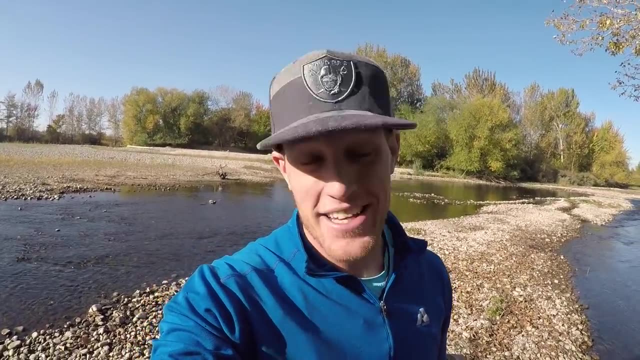 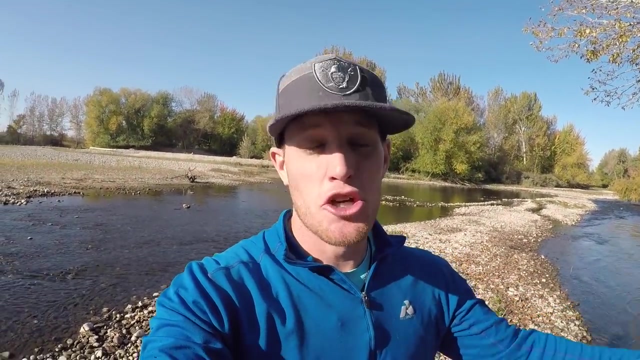 in the stomach: Oh my gosh, Look at that. Look at that fish, though. Oh my word. Oh guys, it looks like they are as aggressive as ever. Let's keep fishing, man, I'm in the same spot. I've literally taken like six casts. I've been here for five minutes. Two beautiful brown 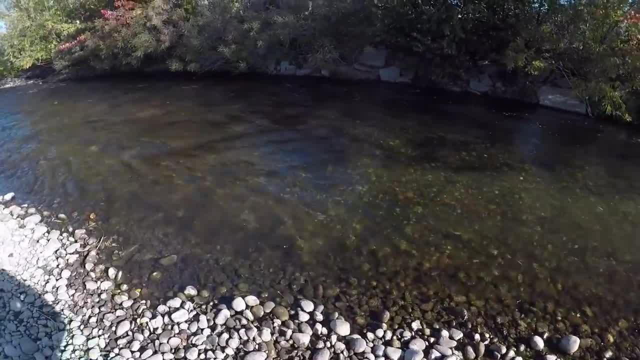 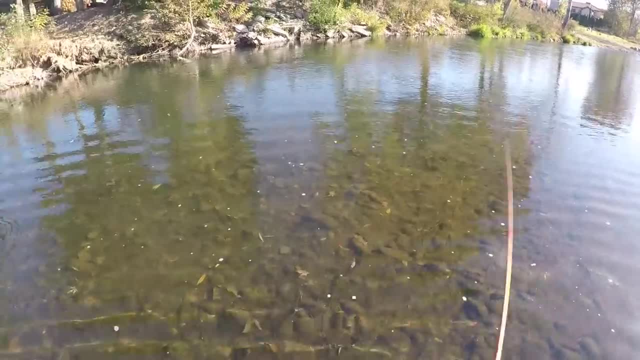 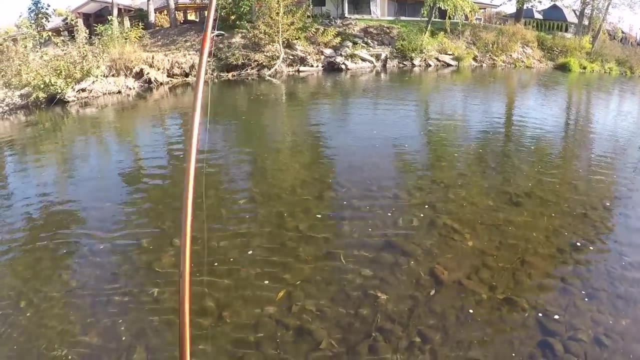 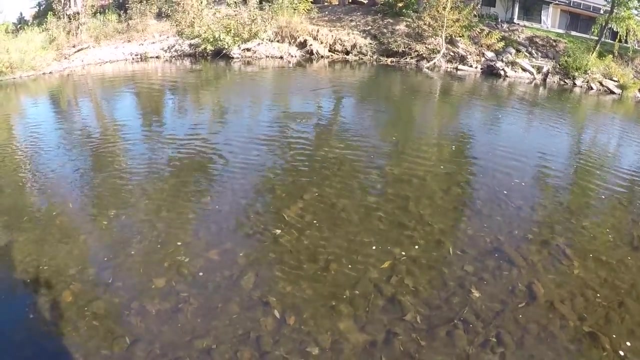 trout already. Let's keep fishing. Big concrete slabs hanging out down there. Oh, there's one, Oh yeah, Oh, this is a rainbow. Look at this, Look at this. Oh, just nailed it, Absolutely nailed it. 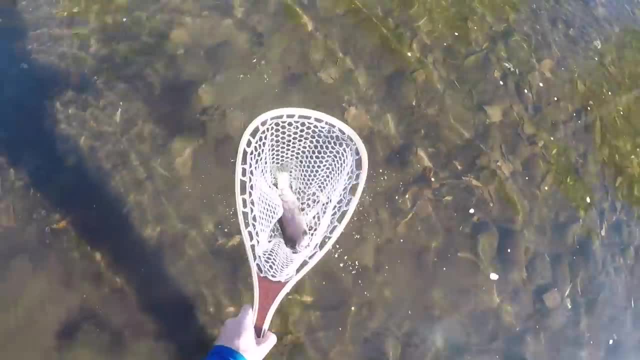 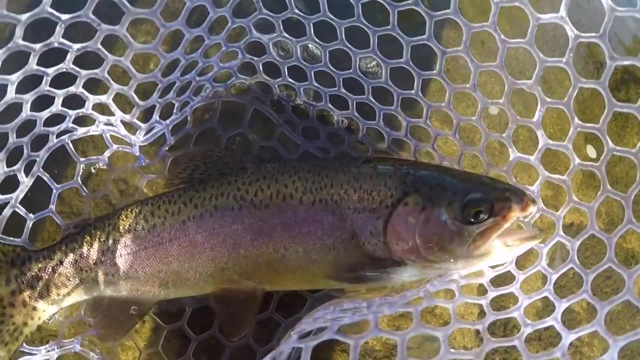 All right, Look at this. Oh, look at that Pretty fish. First bow of the day on that gold color. We're going to keep this one today because I want to throw down a little catch and cook later today. So this is about a 13 inch bow. 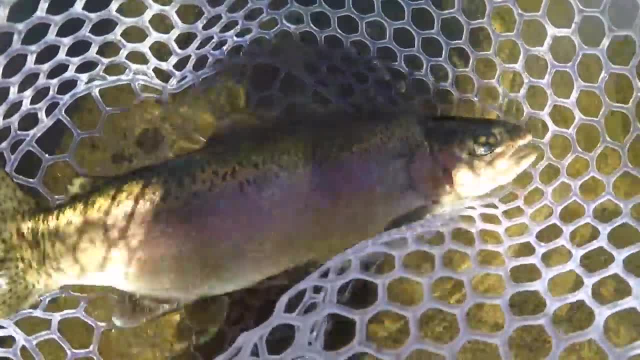 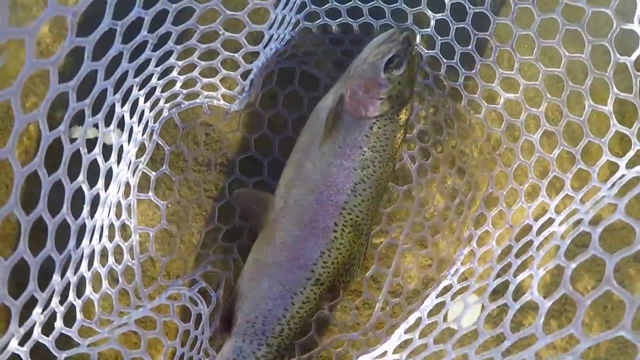 and I'd rather keep a rainbow than those beautiful brown trout. The brown trout are a little bit more rare, So I'd like to leave those in the river, if I can. There are a lot like a ton of rainbow trout in this river, So we're going to keep this guys. We can eat a little something. later I'll show you. 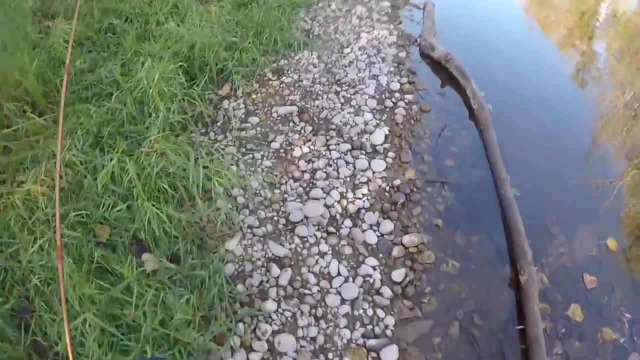 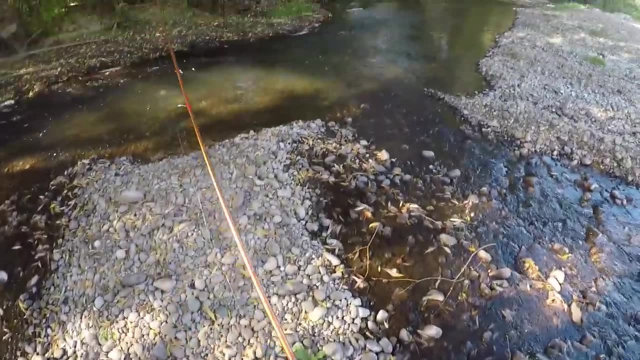 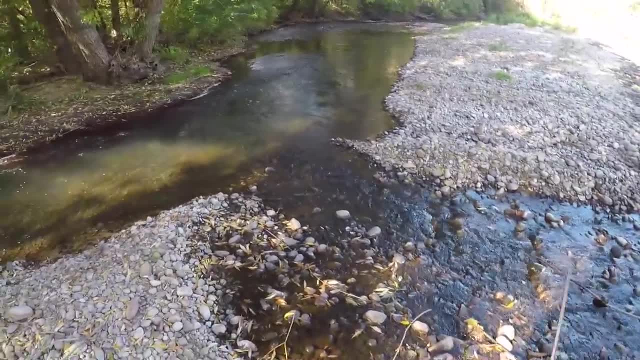 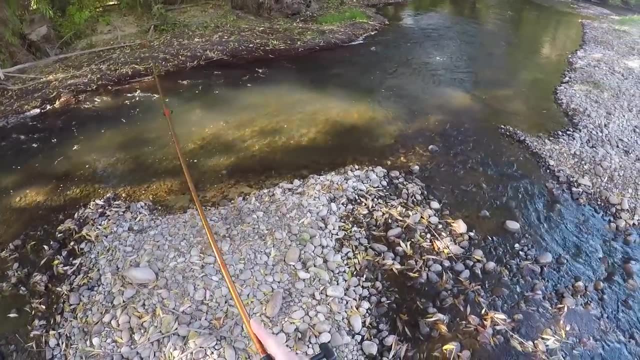 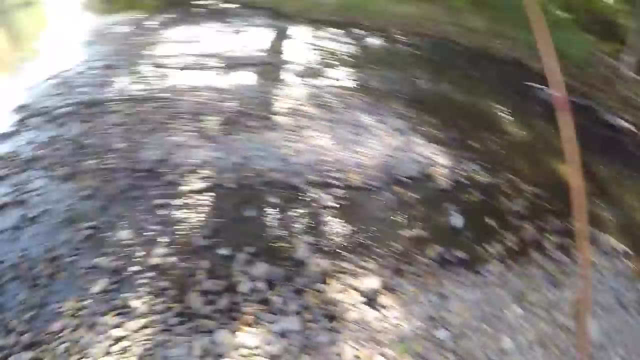 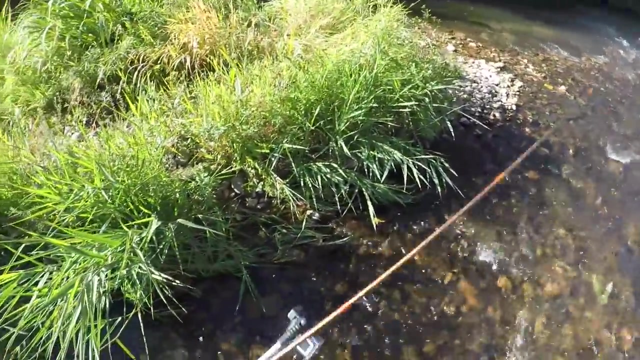 Nice little deep pocket. I don't know Man. it looks pretty good, But looks can be deceiving. Let's move on. Oh, look at this guys. So it just came from up there. Let me set my stuff down here. Got a pitch in here. This looks kind of good. oh, there's one first cast. i can't tell what it is. it is a little rainbow. check it out, look at that. but i can't tell yet smoked it? yep, nice rainbow, look at that. pretty fish, pretty fish, look at that. yeah, i figured it was about due for one. gosh guys, that's three bows now. three bows on the day, add to two brown trout- another pretty fish. guys, this would be a keeper, but i've already kept one. look at that. look at that. get her back in the water. there we go, good fight, boom. that's five fish on the day. rainbows, now, officially, are outpacing the brown trout. that. right in my backpack. look at that. boom. look how small. all right, so set this off to the side. this is super cool. watch this. it just folds out a little cage, drops in the bottom right there to keep it all steady. this can actually go put back up if i want to. close it. so then it's all enclosed, but this is where i feed the wood in, so i set that right there. check it out. there's plenty of ventilation in the bottom because they've got the holes on the sides. you can see me there. oh hello, you sexy stud, anywho. and then it sits just like that, and then 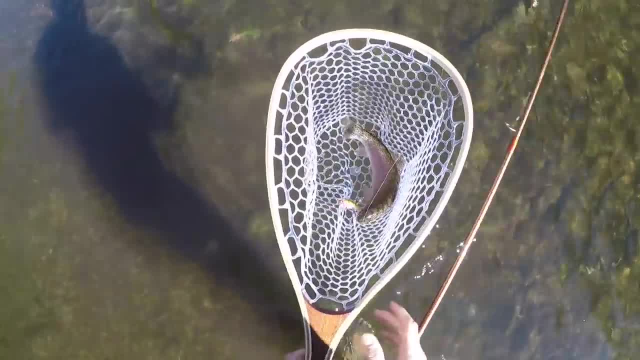 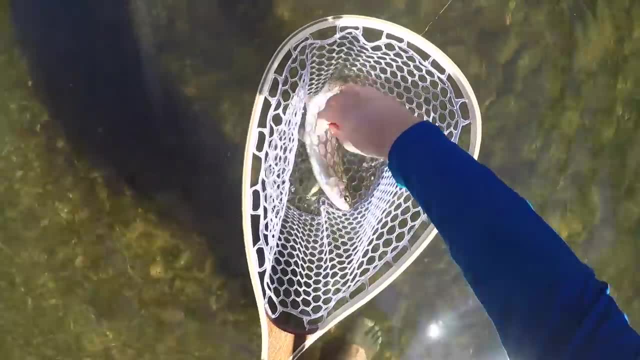 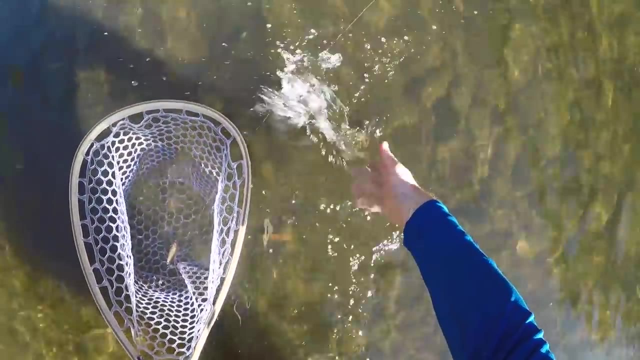 the little grill top: bam, just fits right on top for instant grilling. look at that. this is the first time i'm using it. actually, i found it online and that way it allows me to cook these fish up over an open flame, which is sometimes way more delicious, sir, if that's a word, and i'm excited. i, i'm really excited. so let's go get some wood and let's get a little fire going. now we just start feeding bits of wood in like this. this is exciting. look at that, guys. so all i need to do is make sure to keep feeding wood in through this side. we've got a nice little burma coals built up. we're gonna let that fire die down a little bit, then we will start grilling. all right, look at that. that is looking about perfect, right where we want it. now, guys, today's recipe is pretty simple. i have put a mixture of olive oil and a caribbean jerk marinade- uh, in this little- actually it's a little- wine bottle, but i just tossed the wine out and put this in because it's easier to carry around this way instead of a big thing of a barbecue. So we have a Caribbean jerk marinade and a little bit of olive oil and that's just going to go right over our trout, along with some salt and pepper. There's our piece of trout right there: Nice pink looking meat on the. inside. We're just going to go ahead, set it right there, Go ahead and pour a little of this marinade over the top and on it. What I'll do now is I'll flip it for barbecue in here and over the top. There we go. All right, guys, and I also have the four tails from the crawdad. that I'm going to just toss on there like so We'll drizzle a little marinade over those as well. Got everything barbecuing up, marinating up just nicely. Fire's going good, This is living All right. we're flipping our fish. here. We're going to go ahead and put this on the top. Got a little crispy on that side, but that's kind of how barbecuing goes sometimes. Go ahead and drizzle some more marinade on this side as well. One more time, Let's get into that. fish. Perfect Guys. I'm really excited to give this recipe a try. I've never had trout in a Caribbean marinade, so looks like it's almost done. We're gonna let this fire die down and I'm excited to give this a try, along with some bonus crawdads. It doesn't get much better than this out here on. a beautiful fall afternoon Cooking up your own fresh trout with a few few crawdads. This is living. This is definitely living. All right, that trout definitely got nice and crispy on that grill. Peel that skin back a little bit. Look at that. That's that meat we're. after. right there, I was able to get some marinade in the body cavity, so I know there's sauce all over that. All right, guys, there we go. Smells good Cooked, That's good. That is actually really good. That Jamaican marinade has a sweeter flavor to it, So that goes really well with the trout. You guys definitely need to give this a try. All right, guys, it's part of that crawdad tail, It's it got really charred, so look see how that's just crumbling apart. I wasn't able to control the heat very well and the fish didn't really suffer, but it looks. like the crawdad did. All right, Little piece of meat Definitely cooked through. The crawdad was so cooked it almost had the consistency of jerky but tastes like blackened crawdad. Couldn't really get any of the marinade. I think that all cooked off Wasn't the best You guys know. I'm a hundred percent with you, guys. That wasn't great, but if I were starving I would eat blackened crawdad again. It wasn't terrible, but there are better ways to cook. it Definitely had better. What I am digging, minus the crawdads, is this fish, though, guys. I'm almost halfway through. and this is quite delicious. I should be able to just grab this. Look at that. Peel that whole skeleton right out. Now all I'm left with is that big piece of meat. I'm gonna put a little salt on this, because I put salt and pepper on the. skin, but I'm not eating the skin currently because it's charred, Fresh Flaky Comes right off the skin. Bon appetit, guys. That's delicious, That really is really good. Move to another stretch of river here. So many, so much of this, and 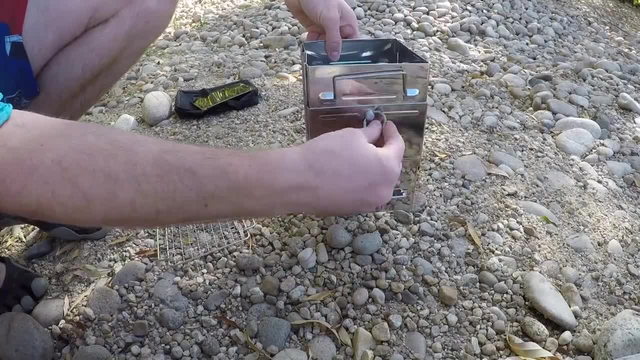 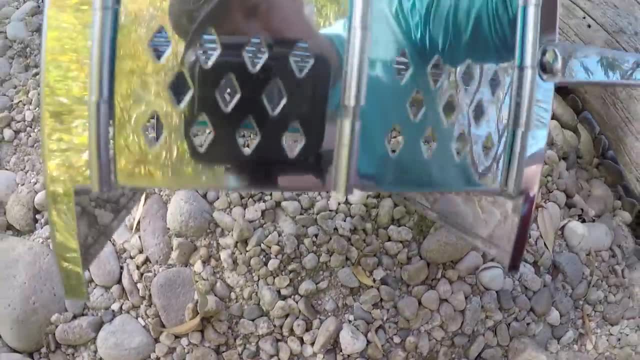 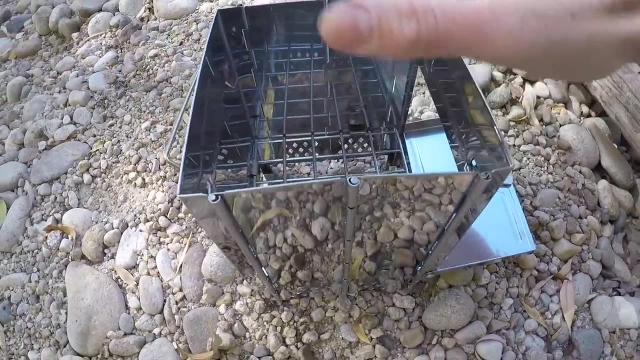 it's a lot of uncharted territory for me still, but those look so good. It's just like man. this looks like there should be some fish holding up in here. Got him. Oh, I felt him load on. I felt him load on. Don't know what it is, but it's. 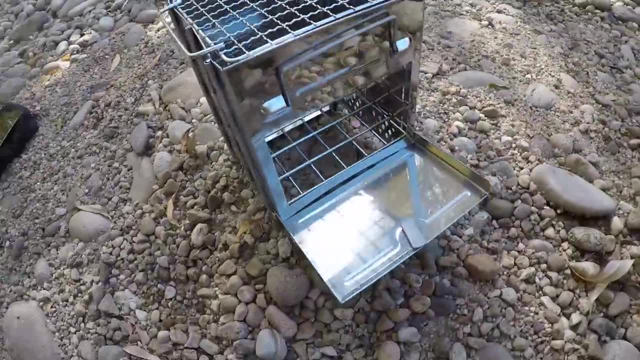 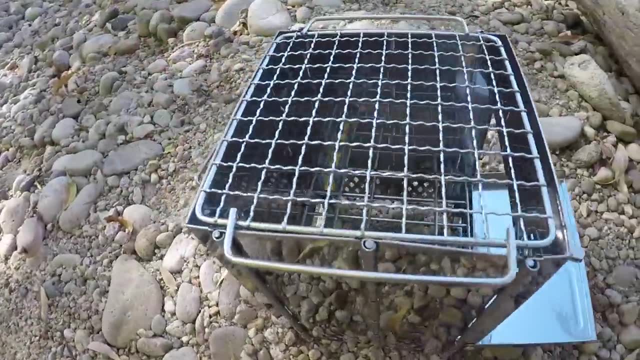 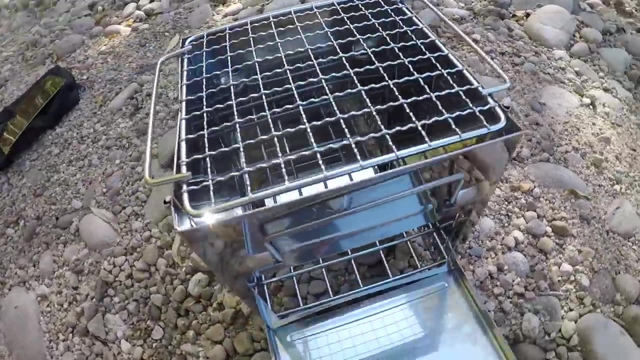 way down there, Guys, on that spinner, On that spinner Between these two fallen trees here I felt him just thump, Thump. I think this is a bow. Nice, Oh, another pretty bow, Pretty rainbow trout. Look at that. Look at that. No, Where you going? 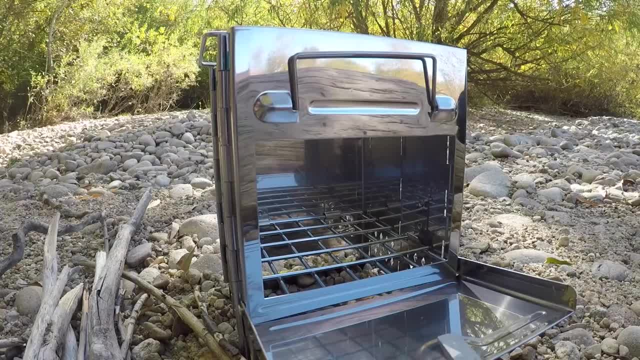 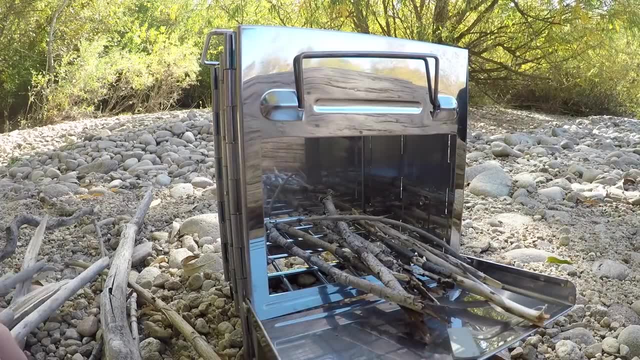 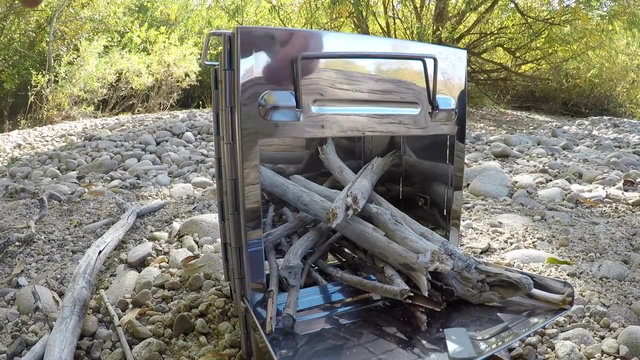 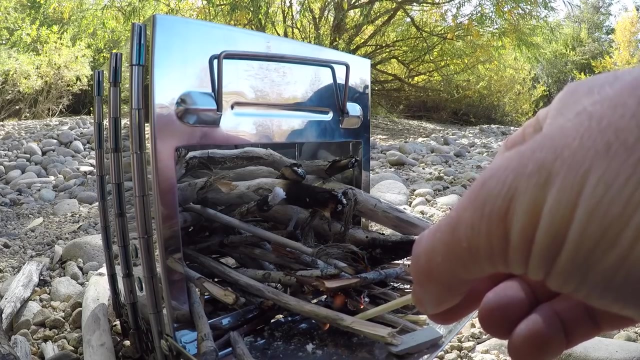 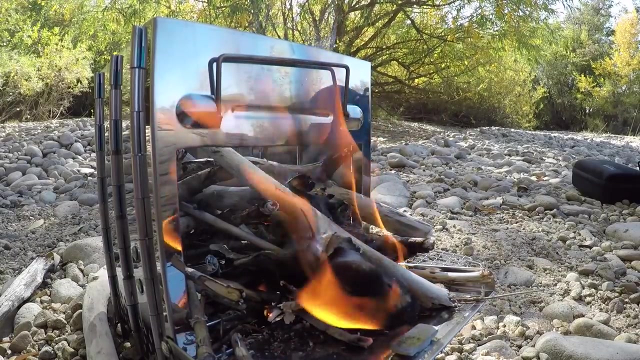 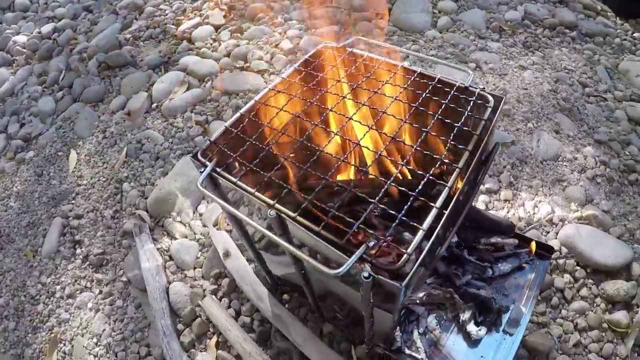 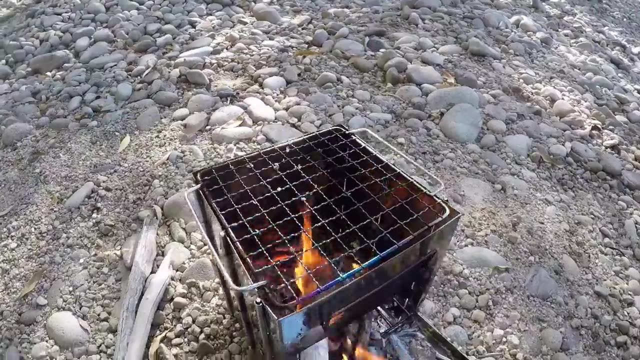 Where you going. Yeah, Nice, Look at that Pretty pretty fish. Sweet, This is a little sketchy, ladies and gentlemen. Ooh, Ooh, Ooh, Okay, Nice and easy. Oh my gosh, There's a little trout Just totally hit the surface right over there. 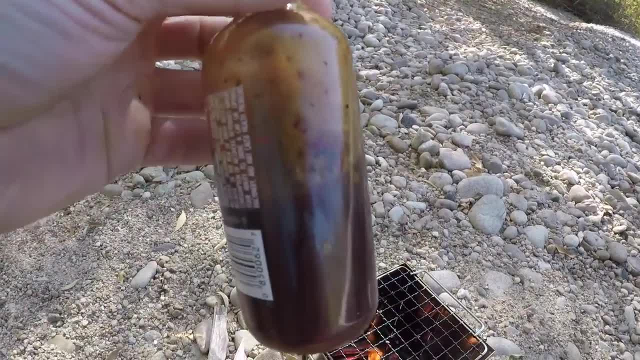 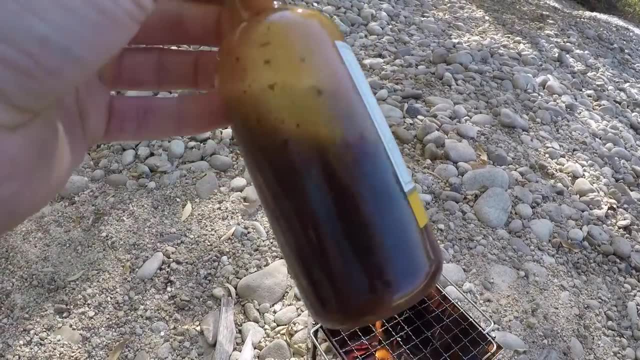 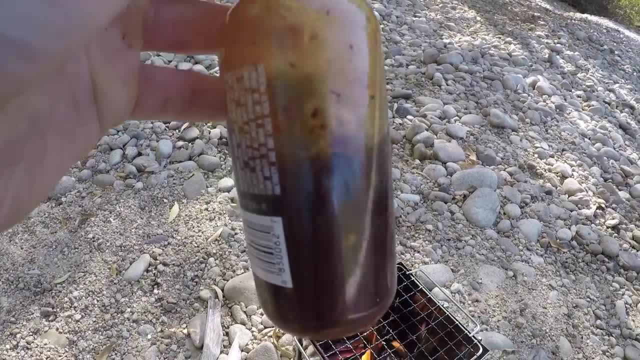 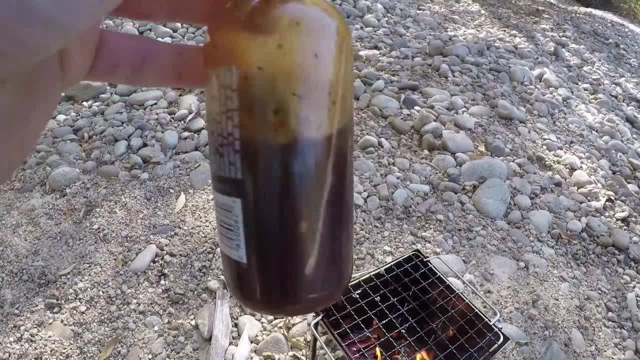 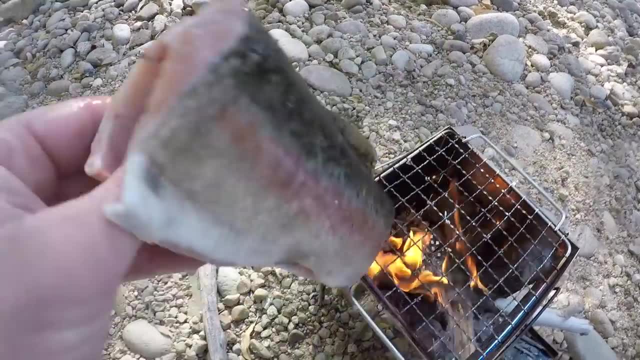 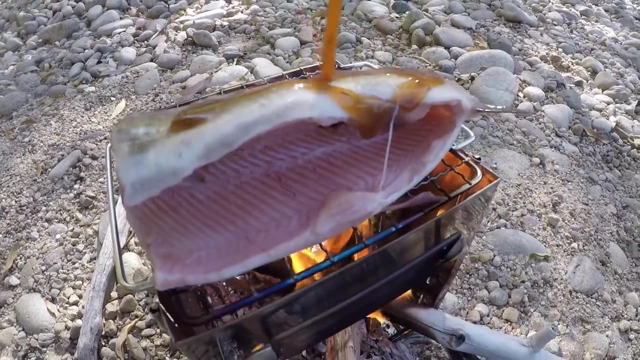 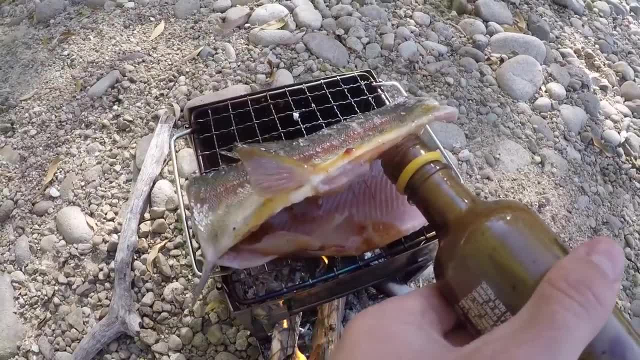 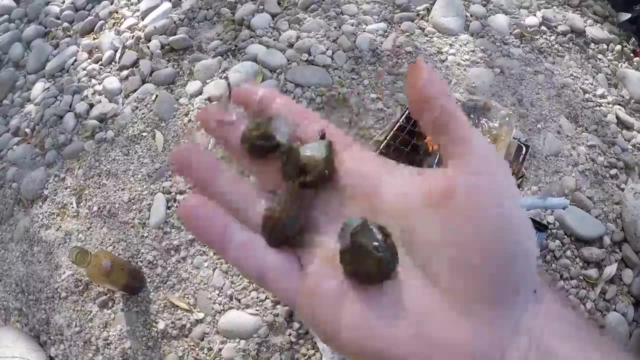 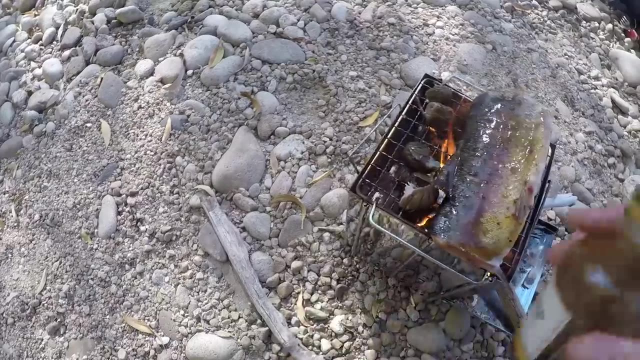 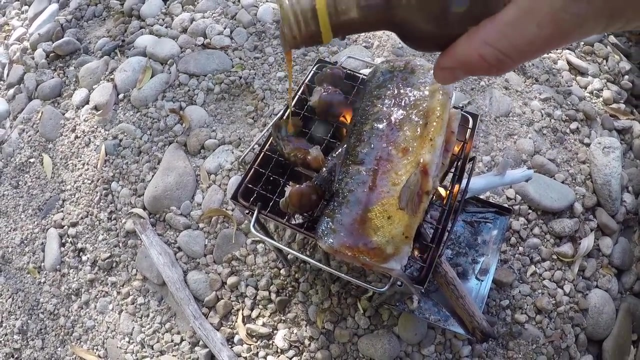 right under that tree over there. I'll bet you that was him. We'll just pop that out, Drop him back in. There you go. You're free to go. Ha ha, Brownie number four Right under those trees Got him. Whoa, That was immediate. Oh yeah, Here we go. What do we have here?